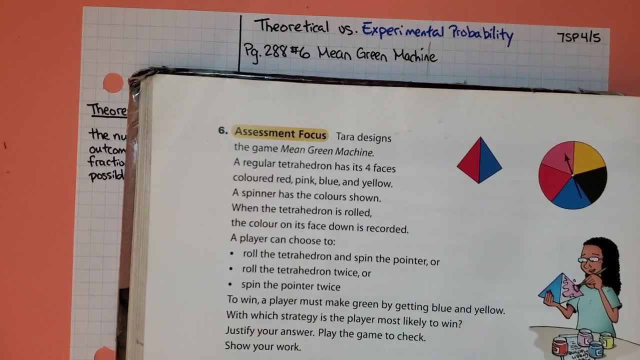 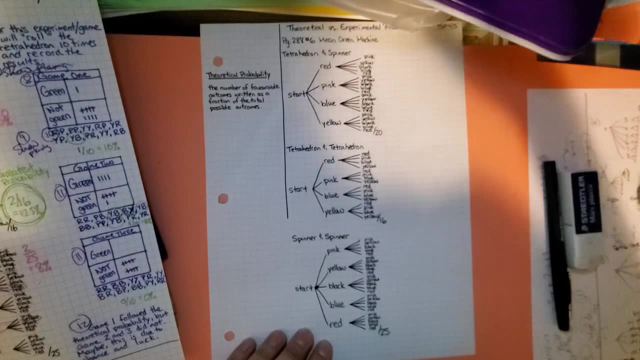 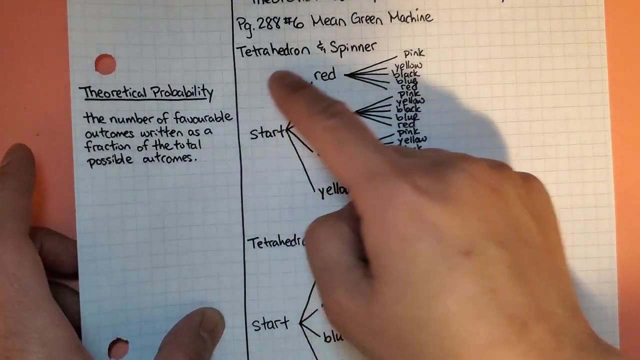 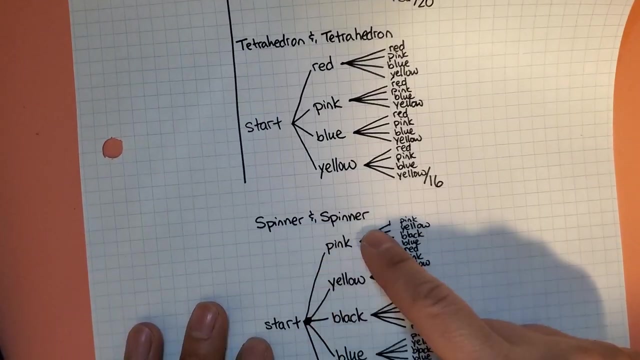 the pointer twice. Alright, so it's blurry, but your sample space should have looked something like this. So, with a tetrahedron, 20 possible outcomes- Oh sorry, tetrahedron and spinner: 20 outcomes: Tetrahedron, tetrahedron 16, spinner, spinner 25,. so the question says: to win a? 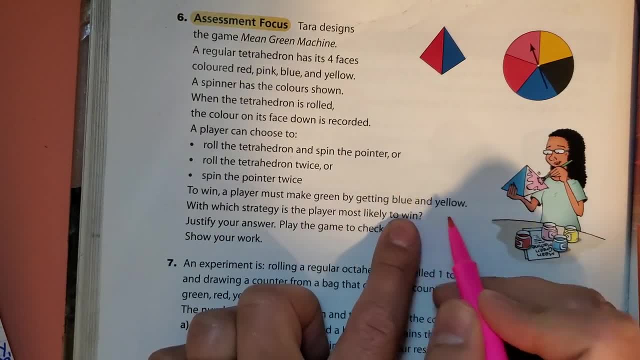 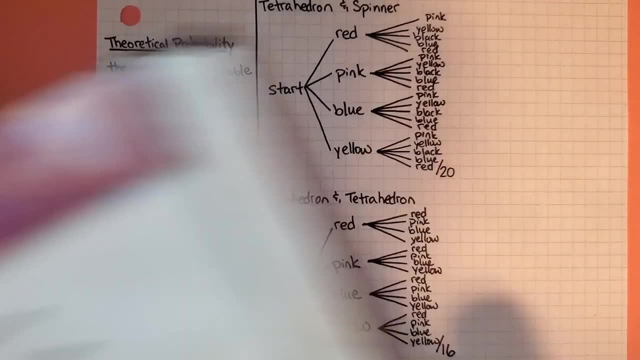 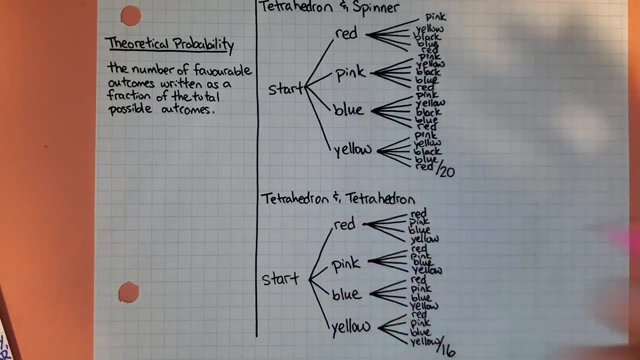 player. a player must make green by getting blue and yellow. with which strategy is a player most likely to win? So after we made all that sample space, we should be able to identify the probability of getting blue and yellow for tetrahedron 60,, 60,, 25.. 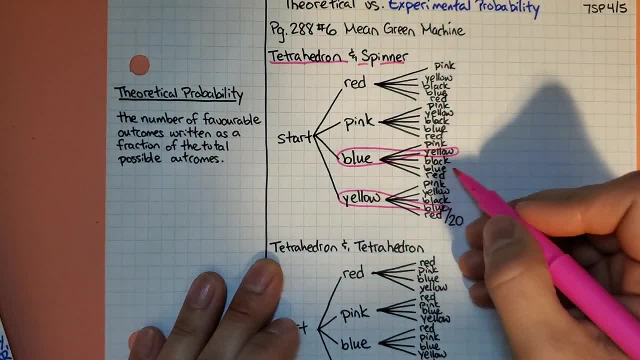 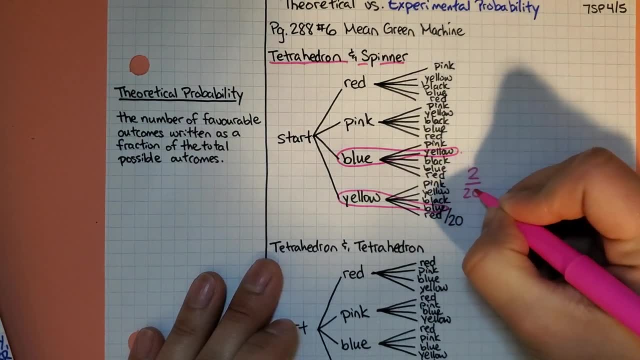 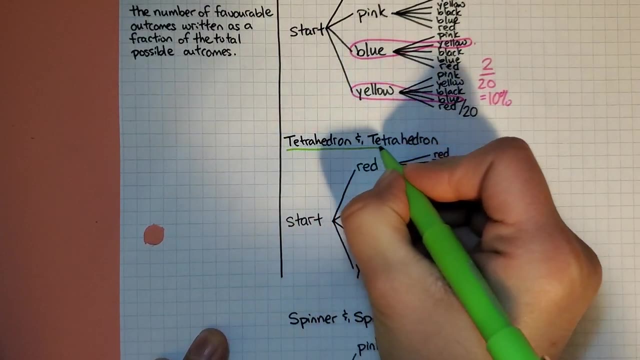 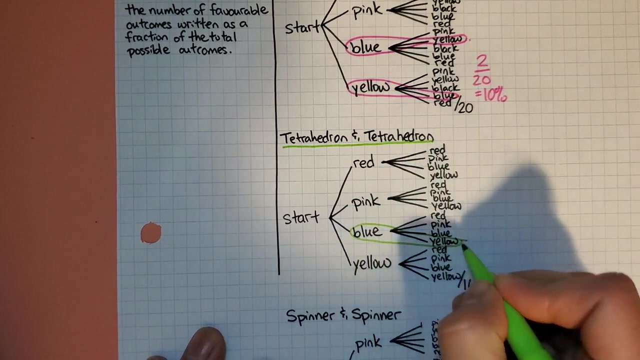 and spinner. the probability of getting blue and yellow is two outcomes out of 20, about 10% for a tetrahedron and a tetrahedron. roll the dice and I roll the dice. possibilities are blue and yellow one time, blue and yellow two times to. 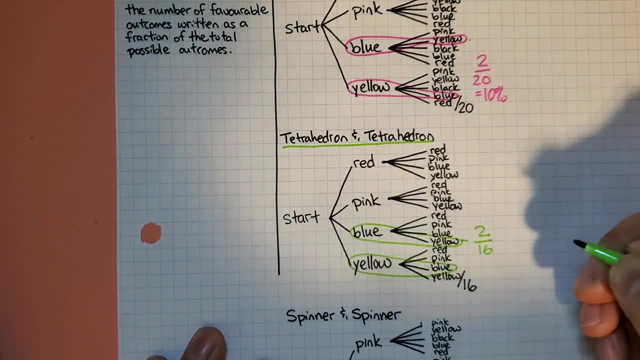 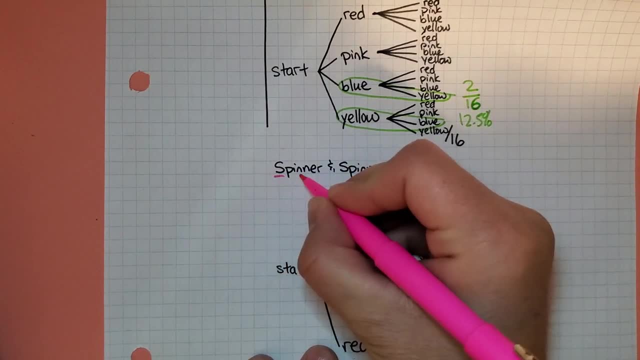 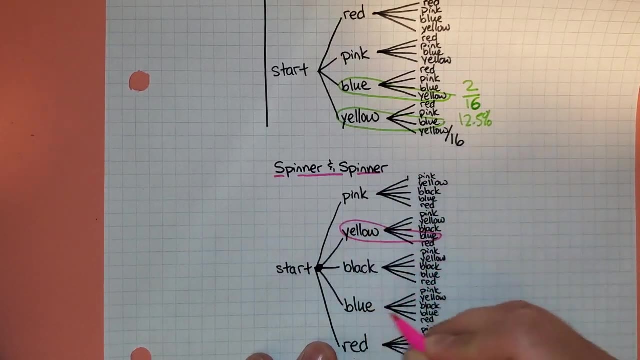 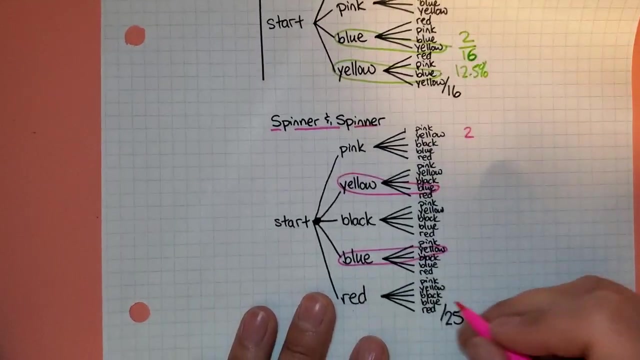 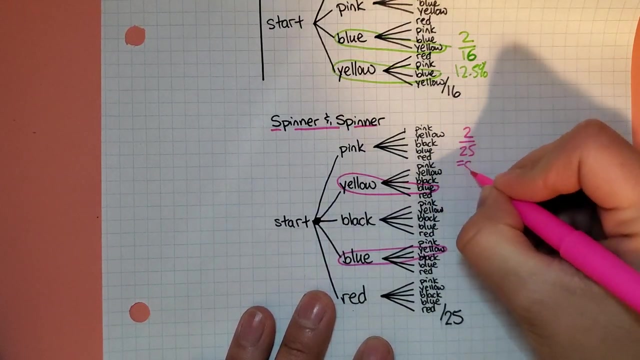 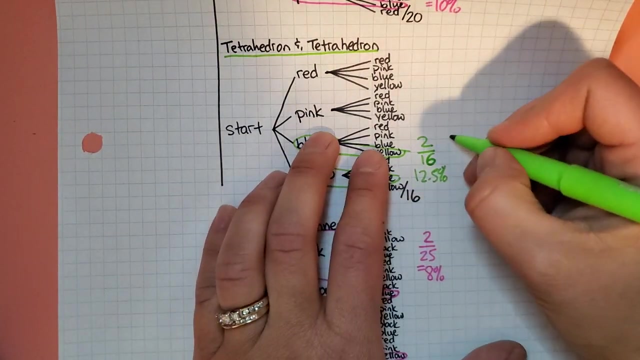 make green. it's a probability of 2 out of 16, which is about 12.5% probability with spinner, and spinner is blue and yellow. blue and yellow is about 2 out of 25. there's 25 possibles, which is about 8%, so the one that will give you about the greatest possibility would be for 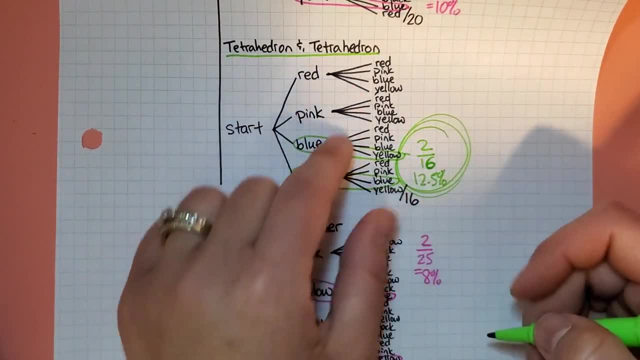 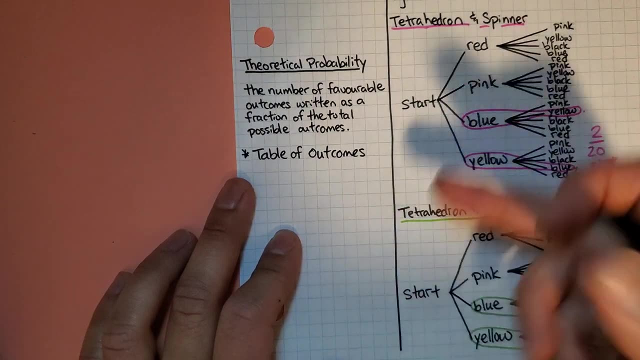 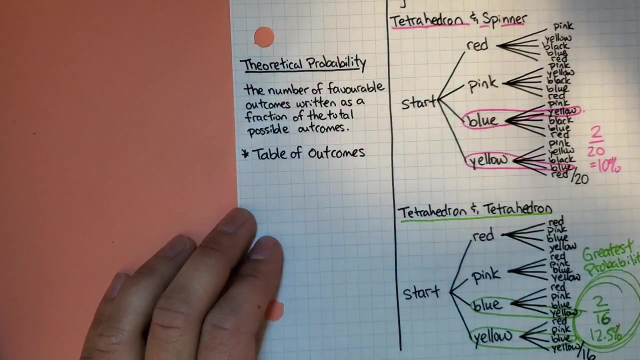 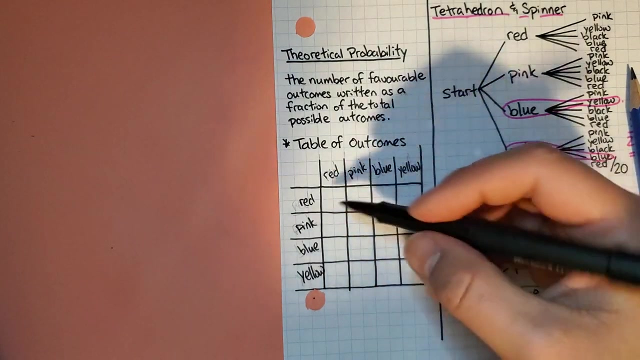 greatest probability getting green is 2 tetrahedrons. last week we worked with tree diagrams. this week again tree diagrams. we can also show it in a table of outcomes and I'll show you what that looks like. so with the table of outcomes you'd list your first roll on the top, second roll on the bottom and then you'd 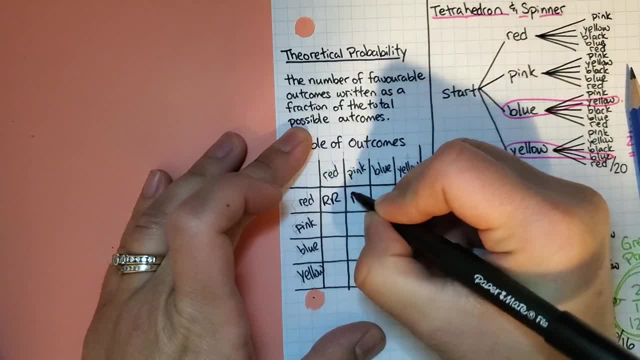 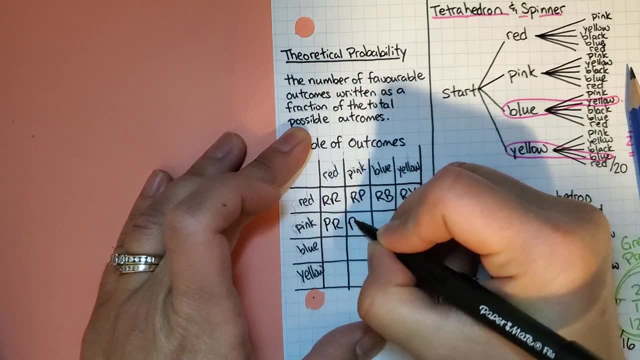 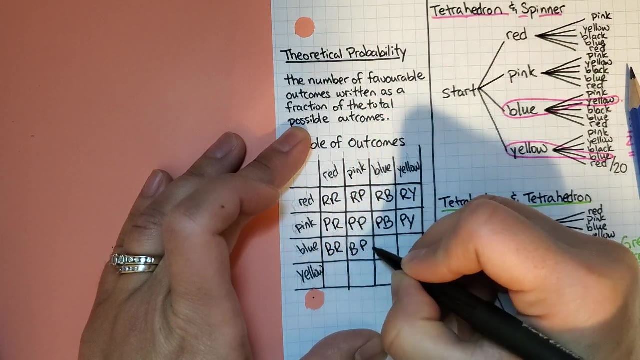 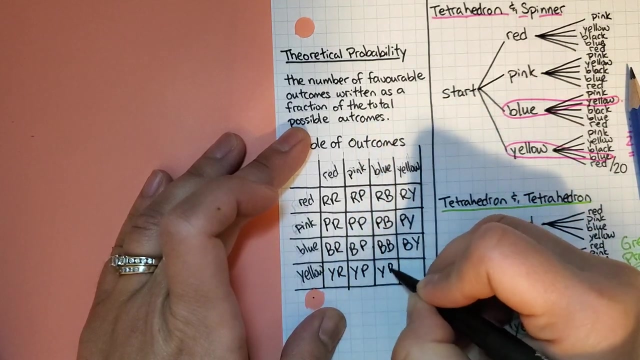 list your outcomes. so here you'd have red, red, red, pink, red, blue, red, yellow, pink, red, pink, pink, pink, blue, pink, yellow, blue, red, blue, pink, blue, blue, blue, blue, yellow, yellow, red, yellow, yellow, yellow. then you look at it and you're like, okay, what are my desirable? 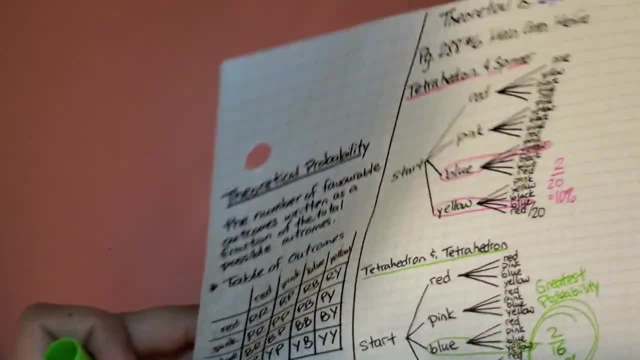 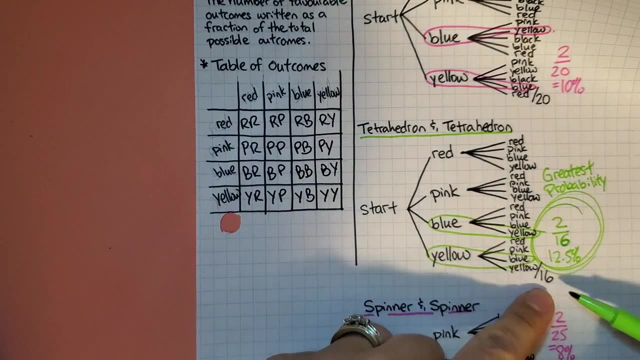 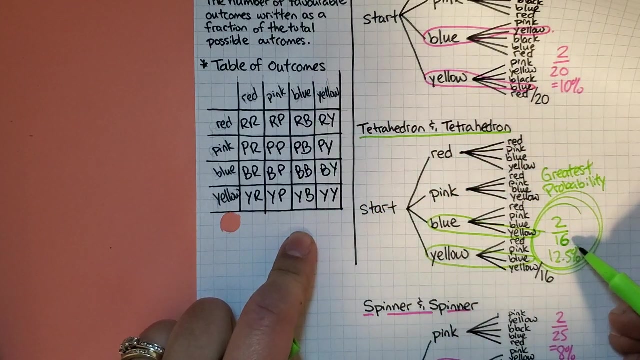 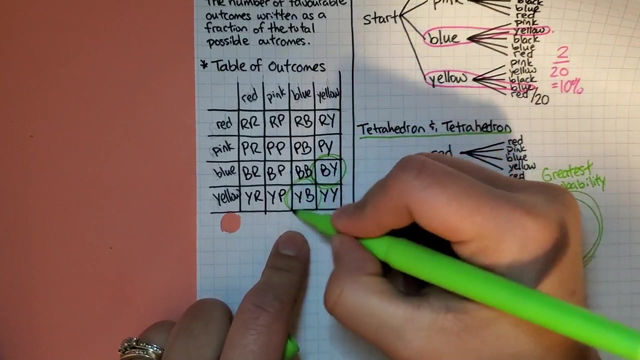 outcomes. and so at the beginning, these two are the same. they show the same things. this one total is 16, this one count them up: 4 by 4, total of 16 and favorable outcomes. same thing: looking for blue and yellow together, blue and yellow together and blue and yellow together: Still 2 out of 16 probability of getting green. 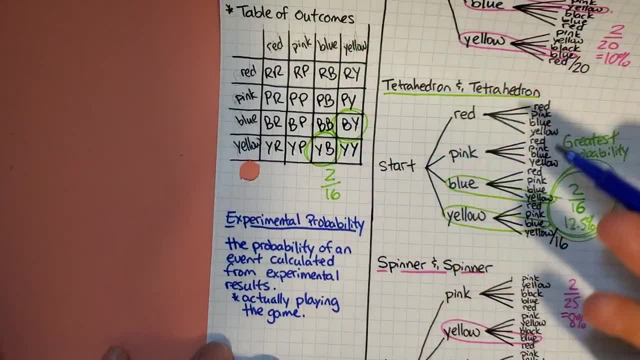 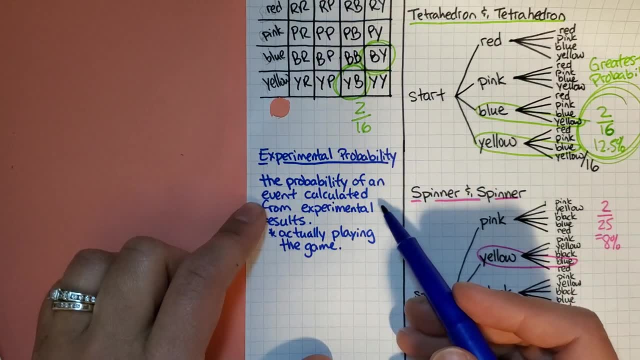 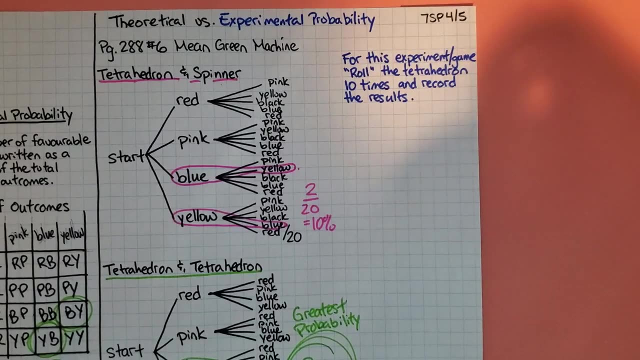 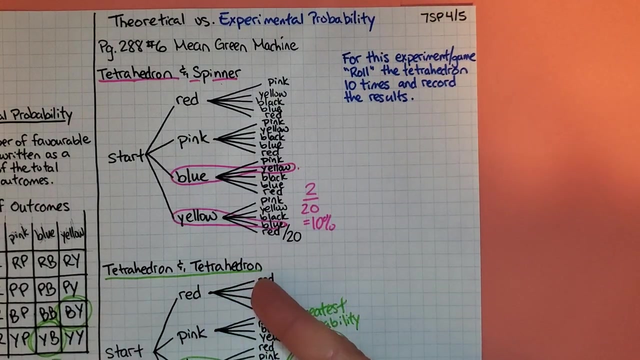 So now, how is this sample space, this theoretical probability, different than experimental probability, Where experimental probability is the probability of an event calculated from experimental results, actually playing the game. So for this experiment or game, we're going to roll the tetrahedron 10 times and record the results. So we're doing tetrahedron and tetrahedron. 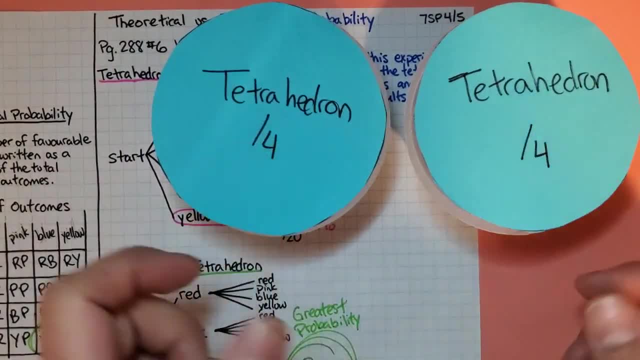 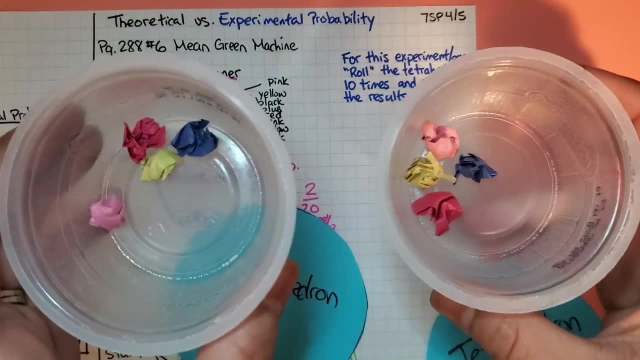 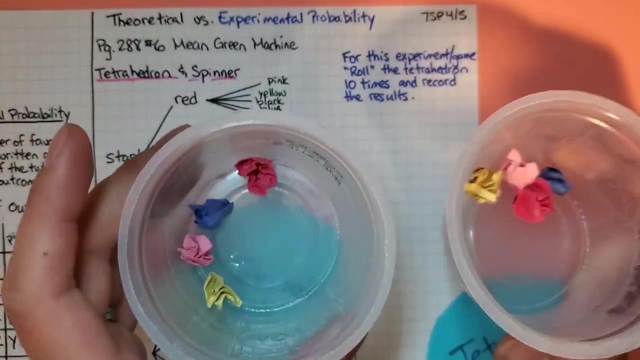 I don't imagine at home you have those, so make your own, just like I'm going to do. Tetrahedron one, tetrahedron number two. As long as you have four equally opportune things or objects or whatever, you can do this game. All right, so you all have paper I took. 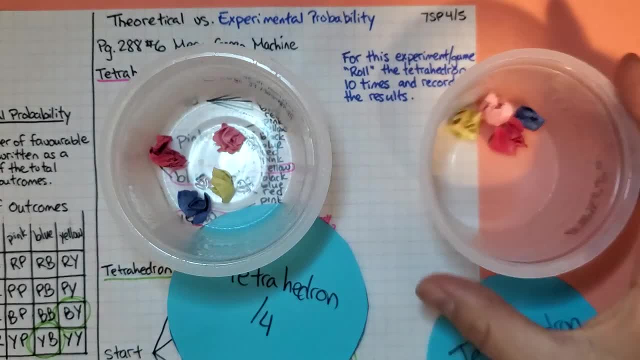 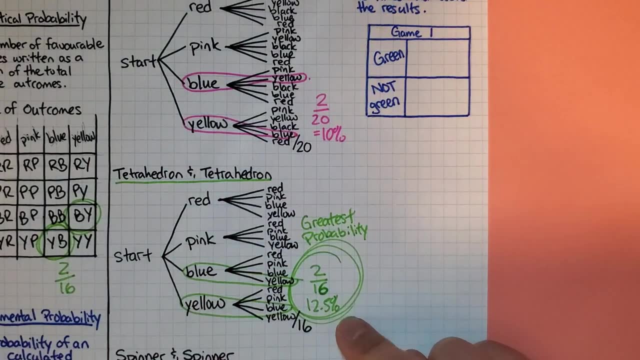 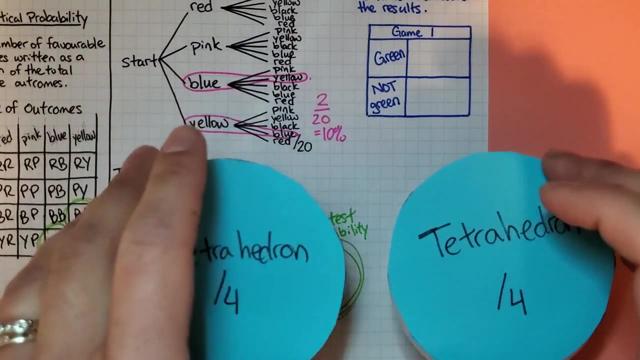 four different colors of paper to make my one dice and the second dice. All right, based on the theoretical probability, we should win. We should get green 12.5% of the time. So let's actually play and see what we get. So I'm going to close my eyes. I draw one. 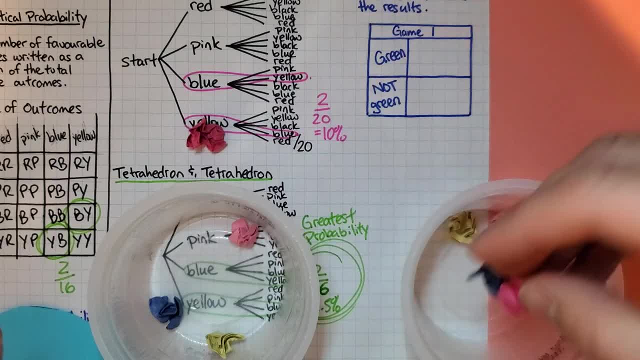 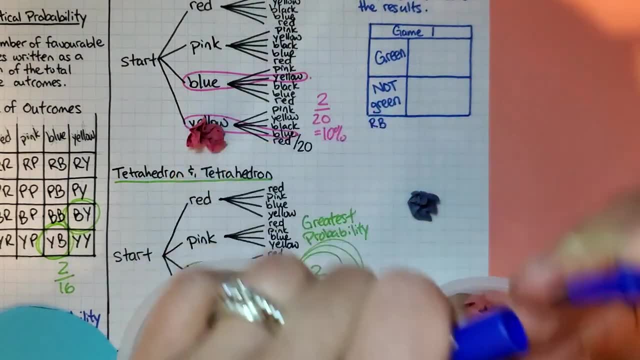 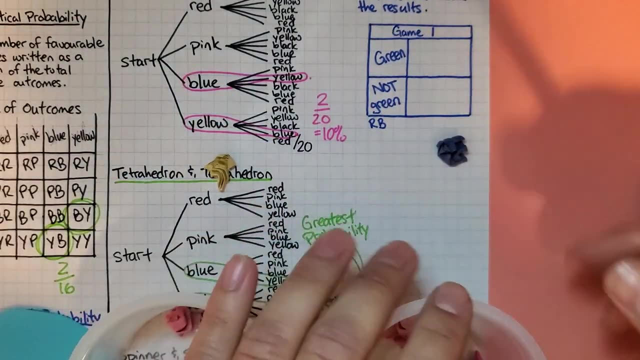 All right, oh sorry, draw one And I draw one. So I get red blue. So I'm going to record my results right here. Red blue: Okay, I'm going to do this 10 times, One from each. Oh, I got one Blue yellow. 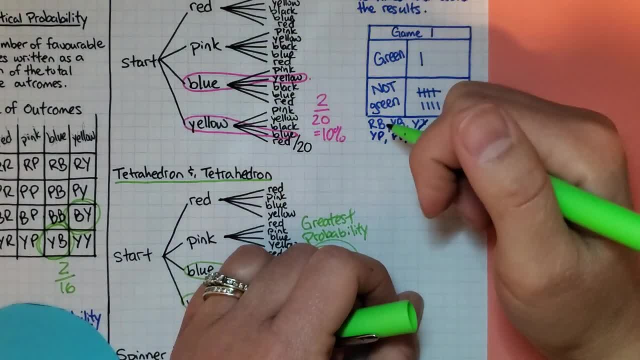 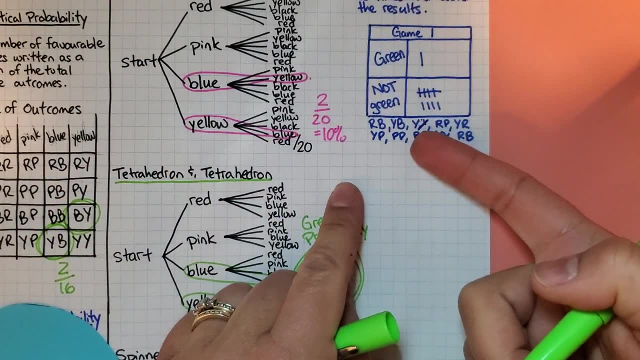 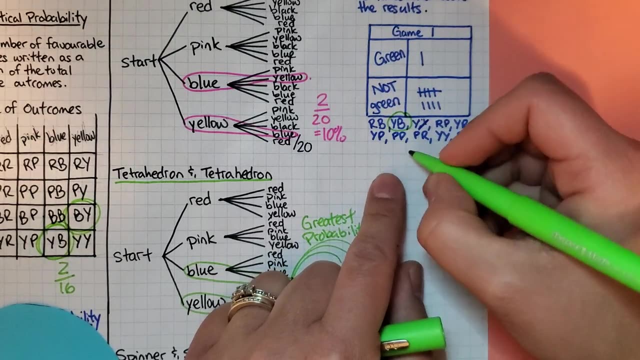 All right, and I'm gonna do that 10 times. So I recorded my results after I rolled- rolled air quotes the dice ten times. I only got green one time out of that whole ten times. So my experimental probability is one out of ten. 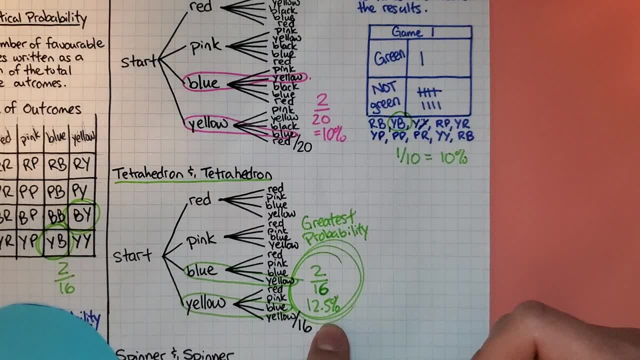 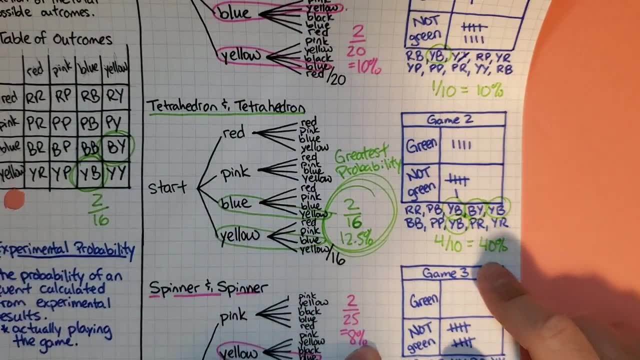 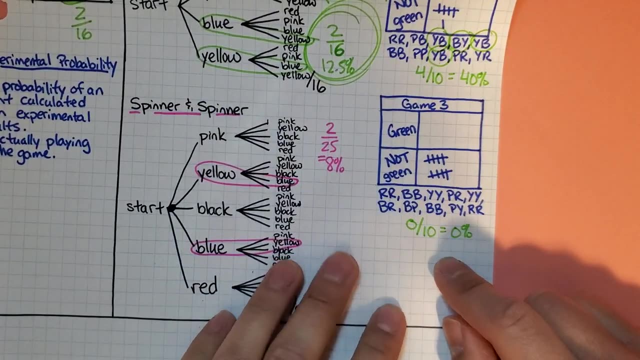 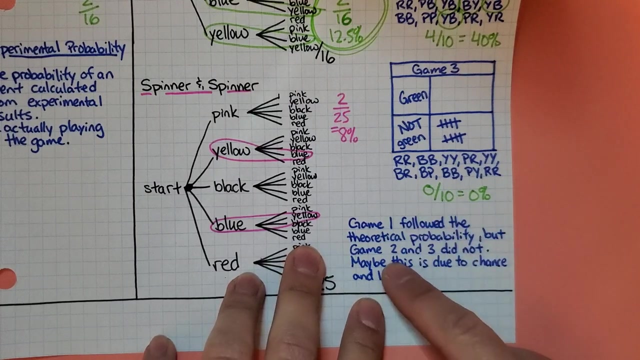 Which is pretty close to my theoretical probability. I'm gonna play this game two more times. In the second game that I played, ended up getting green four out of ten times, And then in the third game that I played, I got 0 out of 10 for making green. So from our experimental 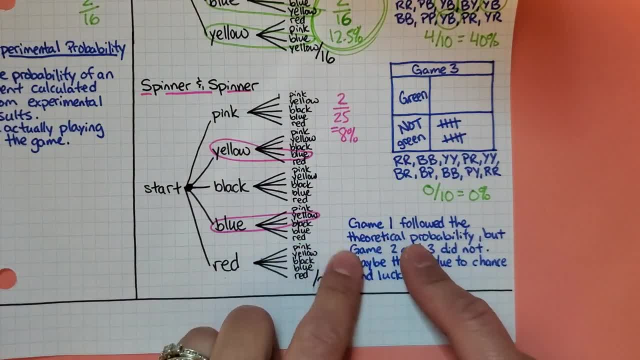 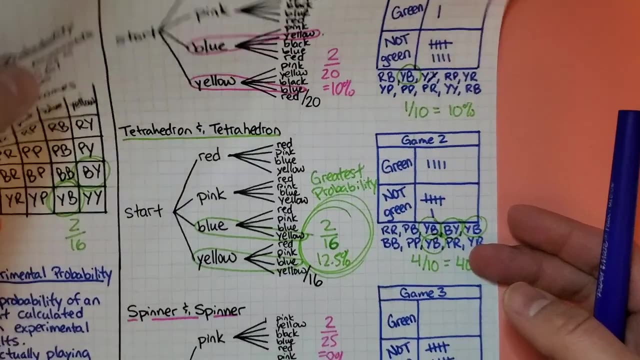 probability results. we found that game 1 followed the theoretical probability, but game 2 and 3 did not. Why is this? Well, maybe this is due to chance or luck. but that's the joy of the experimental probability. It's a little bit different. 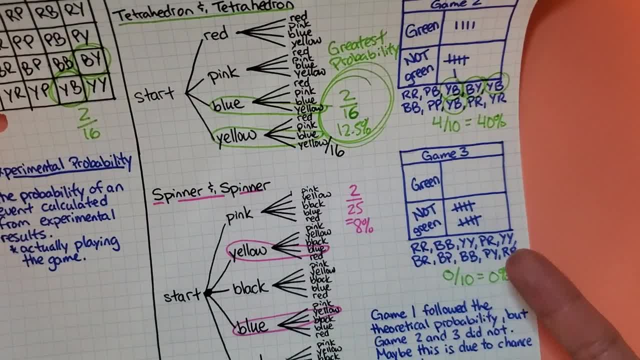 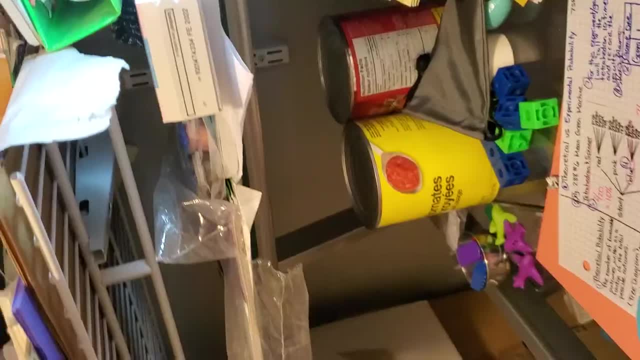 every time. Theoretical, never different, Experimental sometimes different. Let me know grade 7s if you have any other questions. Peace out. 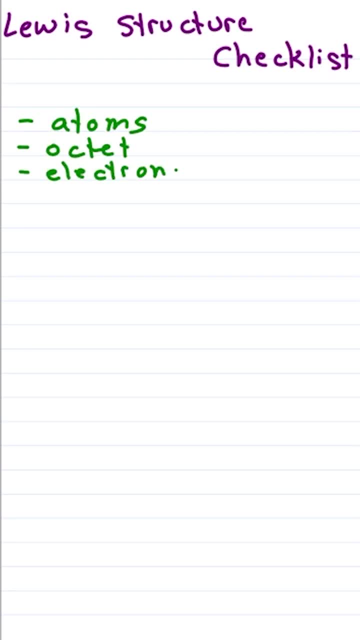 This Lewis structure checklist will not only save you time, but catch any mistakes before you're done. It's different from what your professor teaches, but I teach you to be right. Nitrate, NO3- Nitrogen, least electronegative in the center surrounded by oxygen. 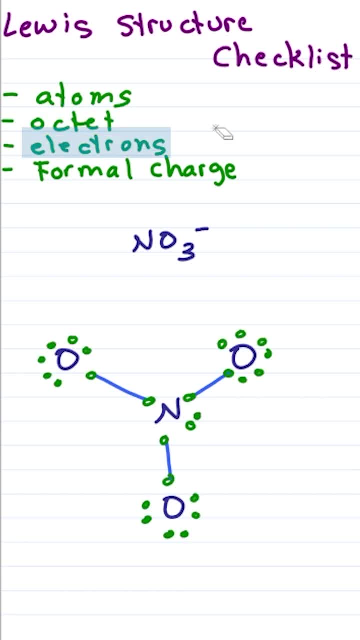 Give every atom a complete octet. This is where we catch if we have too many. Nitrogen has 5.. Oxygen is 6, times 3 is 18, plus 1 for the negative charge. We should have 24 electrons: 7,, 7,, 7, and 5, for a total of 26,, when I should have 24.. 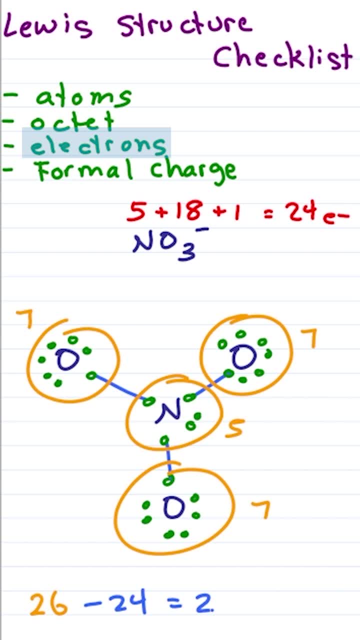 And here's the trick: Take the difference to see how many extra you have, and for every 2, cancel out neighboring lone pairs and put a pi-bond between them. In this case, I'll cancel a lone pair from nitrogen oxygen, put a pi-bond between them and a recount gives me 24..